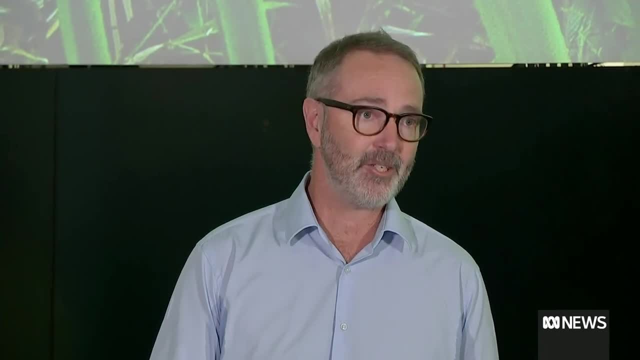 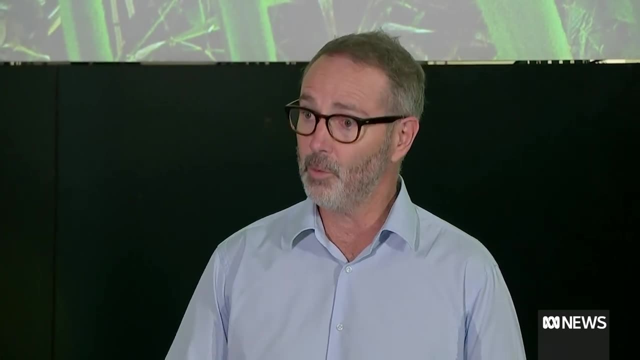 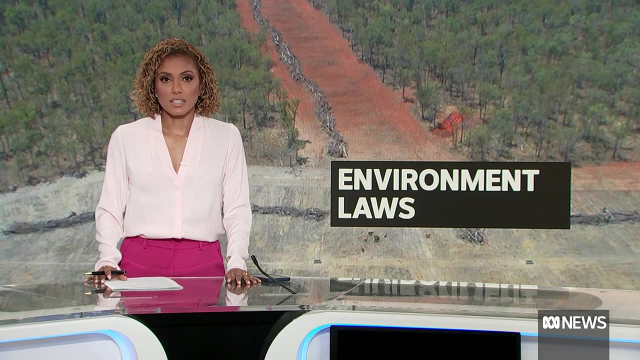 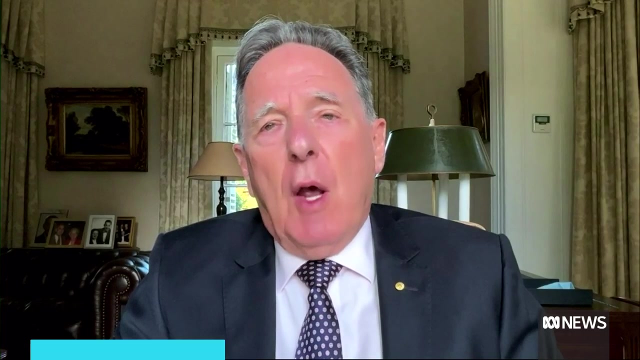 the first in this country's history, and to strengthen our national environmental standards, to establish new standards that will drive this law forward to protecting the environment. Professor Graham Samuel authored the review. Thank you, We've waited so long for this, but don't worry about my view. Think of those that contributed. 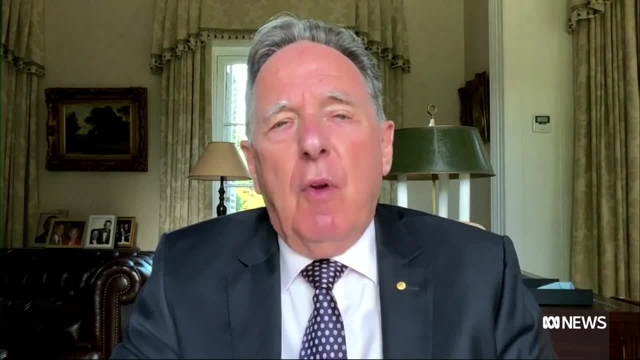 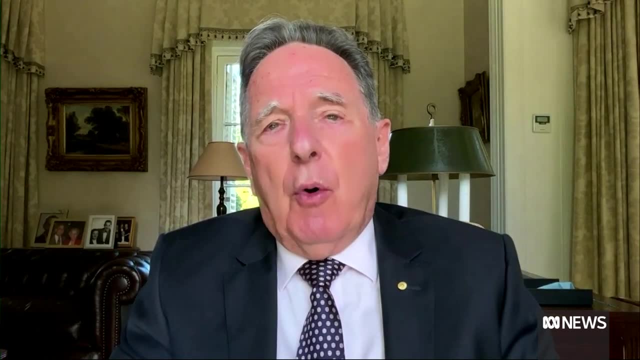 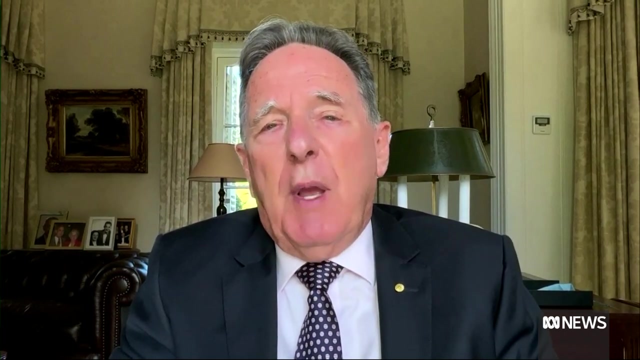 to the review itself. Academics, scientists, business, farmers, conservationists, First Nations people- Right across the board we had people who were terribly concerned about the environment. There are 2,000 threatened species that have been on and off the ground. 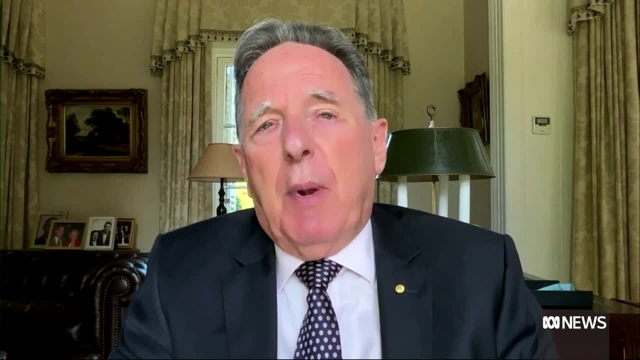 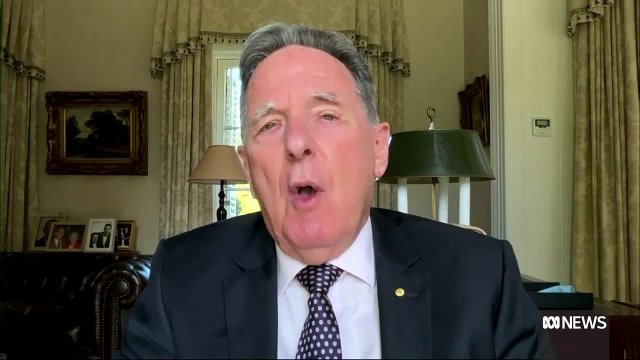 They've been on a list for so long and no recovery plans in place or being implemented to deal with them. All of those parties, including the 2,000 threatened species, ought to feel very satisfied. I've got unqualified admiration and respect and appreciation for what the 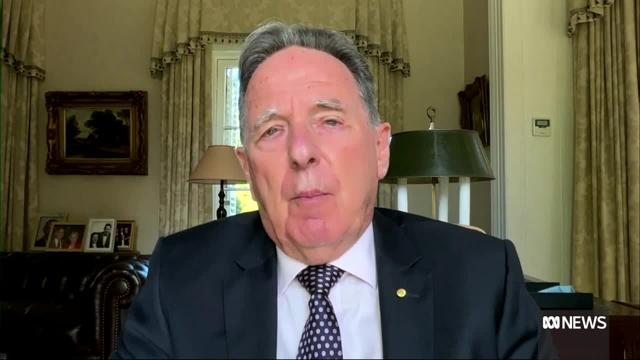 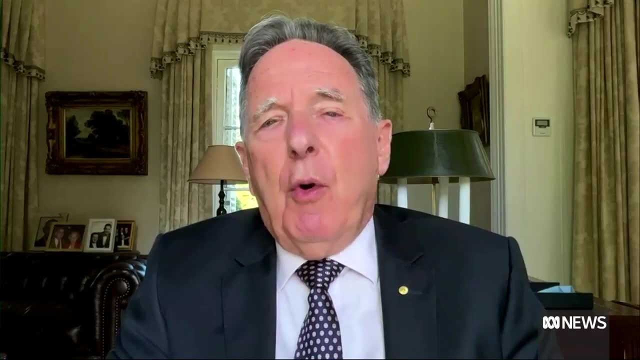 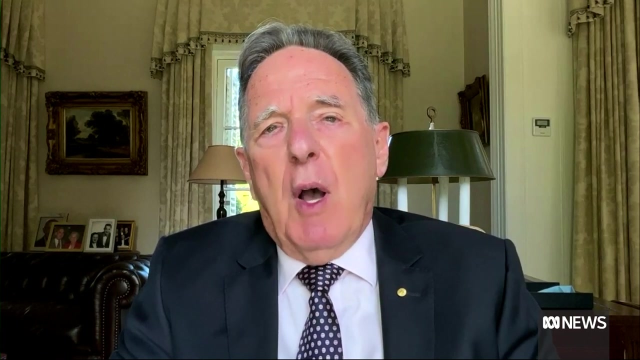 minister has done in the response to the review? What will the establishment of a federal environmental agency make? It's very important Not only to ensure that what we have is safe, but also to ensure that what we have is independent enforcement of the environment laws, but also to oversee. 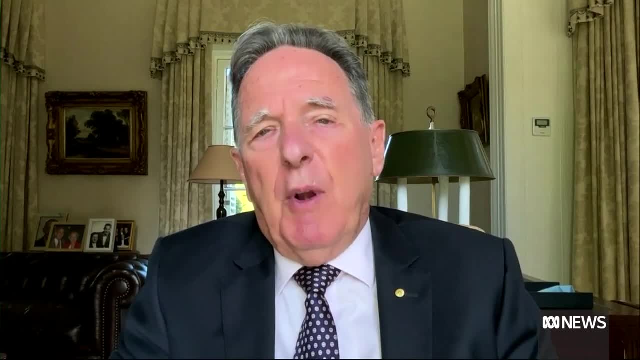 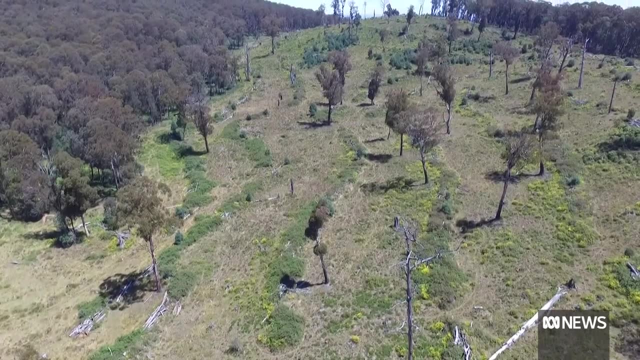 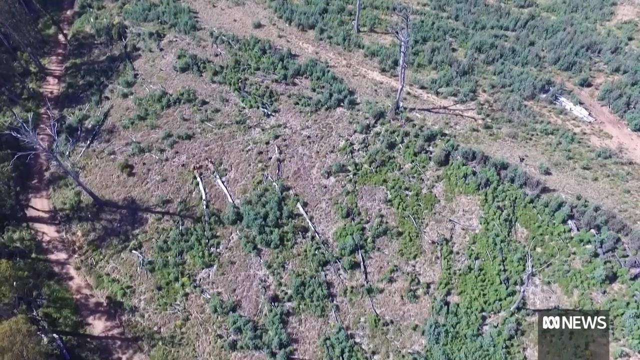 the accreditation process that's proposed in the minister's response. It's an accreditation process that will facilitate more efficient decision-making in respect of applications for developments and the like that have an impact on the environment, But that accreditation, which will go through to states and territories, needs to be overseen by an independent agency. 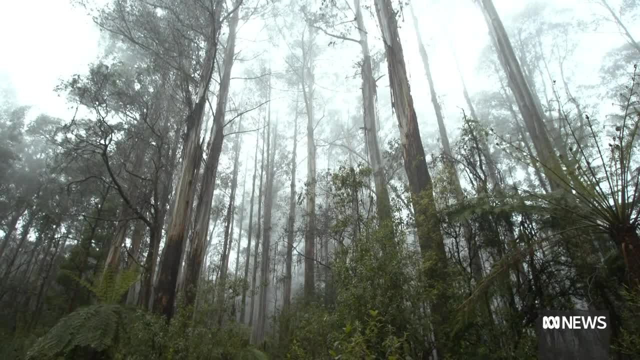 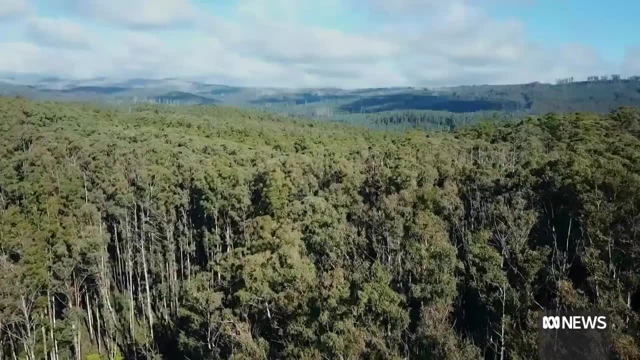 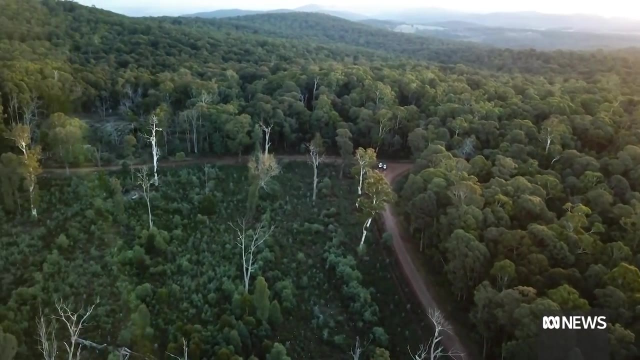 such as the Environment Protection Agency proposed- Thank you- So that states and territories abide by national environmental standards that the government will introduce as part of the law, and those environmental standards will ensure that the right level of environment protection and biodiversity conservation is put in place. 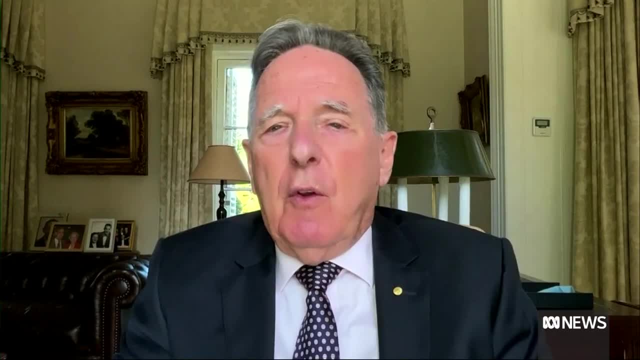 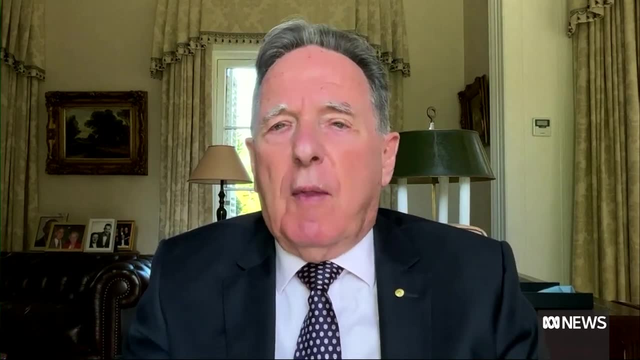 and cannot be allowed to be compromised by some of the other tensions that apply in this area, tensions such as mining royalties, political issues and the like. The minister has properly seen that. He has said this: Environment Protection Agency will be completely independent of government. 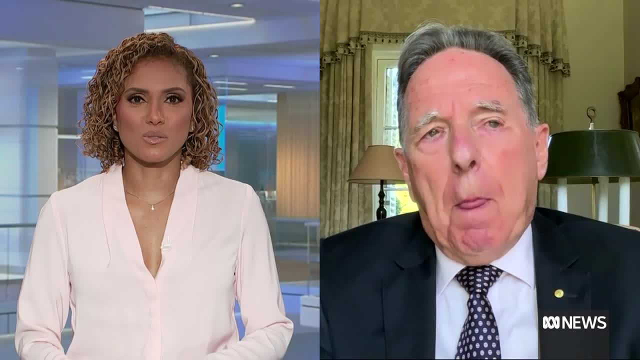 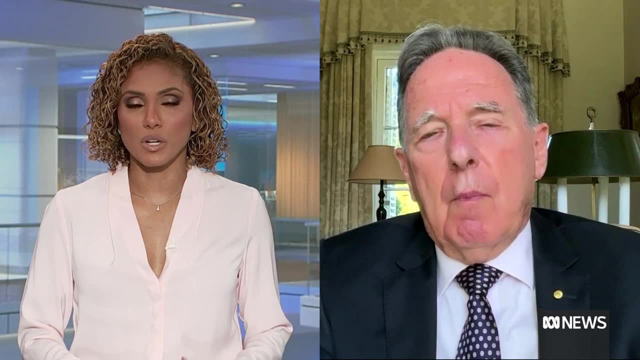 and of politics. OK, you talk about tensions there. One of the criticisms of your review is that it doesn't include a climate trigger, a mechanism which would force regulators to take account of emissions when approving projects. Why didn't your review include that and would? 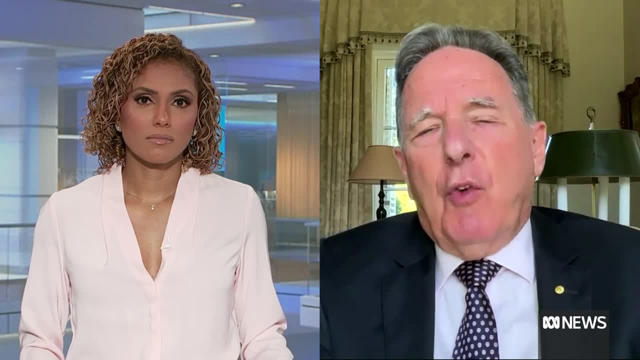 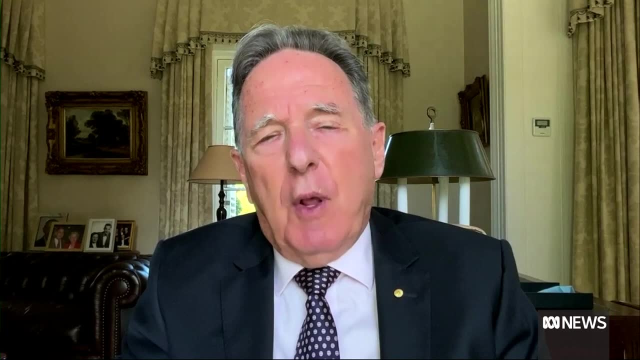 that be a logical next step. Well, I think there's two comments to make. The first is that the view I took was that climate was such a complex issue, It was dealt with by a different minister, by a different department and has different laws, And so it seemed to me that that was the better. 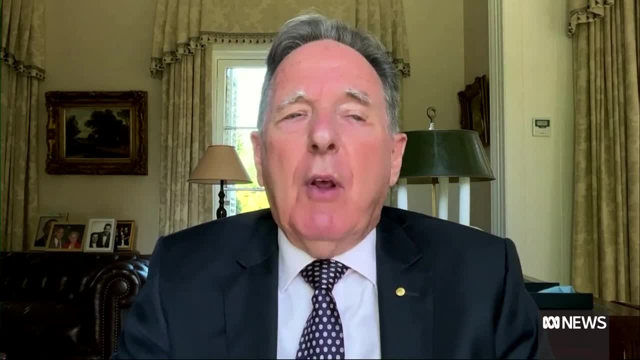 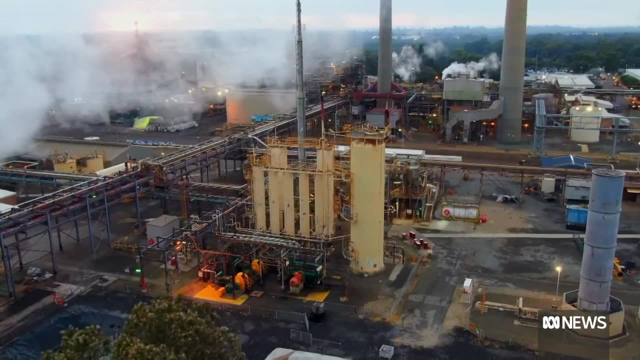 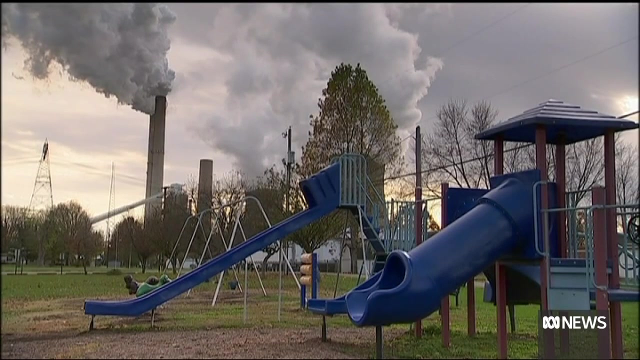 place for these to be dealt with. But- and this is the important but- recommendation: two of my review recommended that all applications for development for mining, whatever it might be needed, to be subject to a complete, transparent disclosure of the impact on carbon carbon. 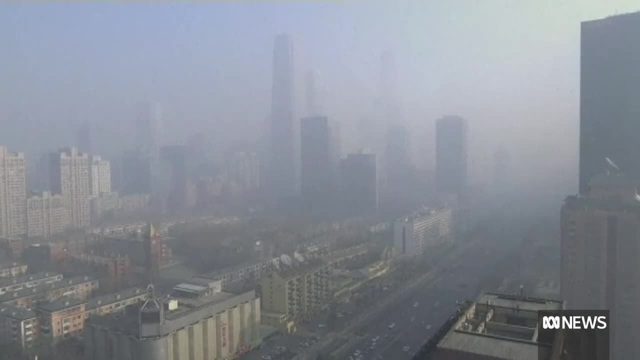 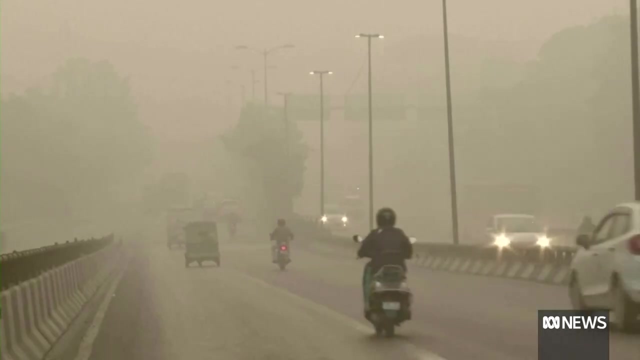 sink, carbon sequestration, and what steps were to be taken by the proponent of the bill, the representative of the development, to mitigate that impact. Now that recommendation has been adopted by the minister, Transparency is a very important element here, and one. 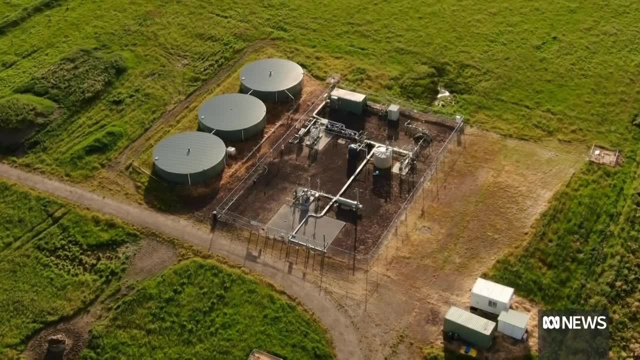 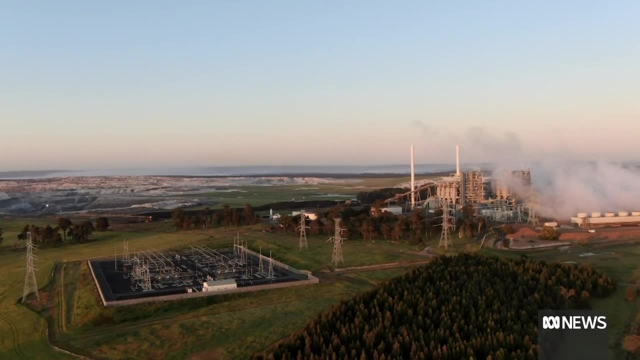 could contemplate that those sorts of issues will be taken into account in determining environmental approvals? Graeme Samuel, very quickly because we're running out of time: your review recommended federal powers of approval be handed to the states, but that was rejected by the environment. 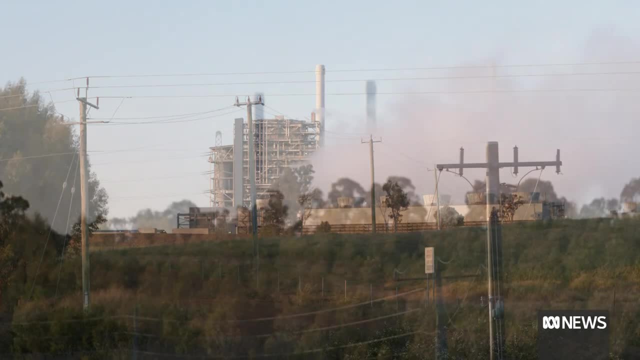 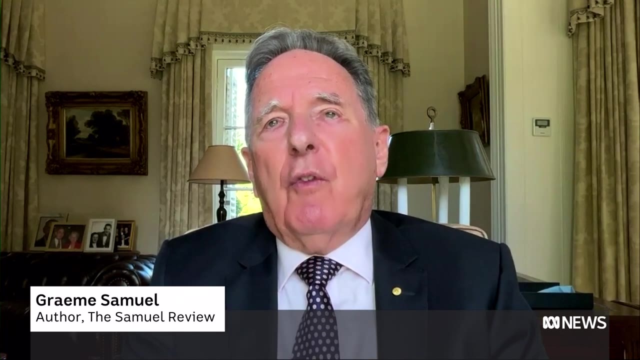 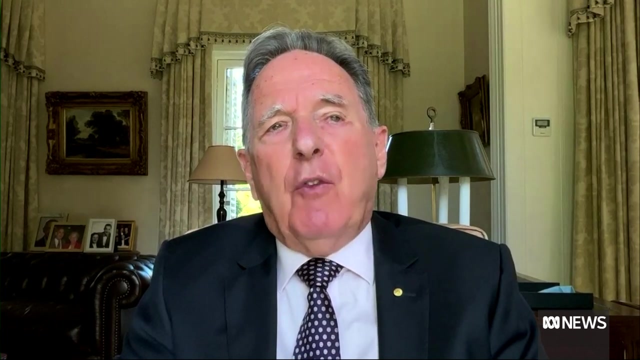 minister? Was that political in your view, given that transfer of responsibility? Was that in line with a long-held coalition policy? Well, I think that what's happened is that the minister has said that some elements of accreditation will take place, but- and this seems very important- they'll be subject to. 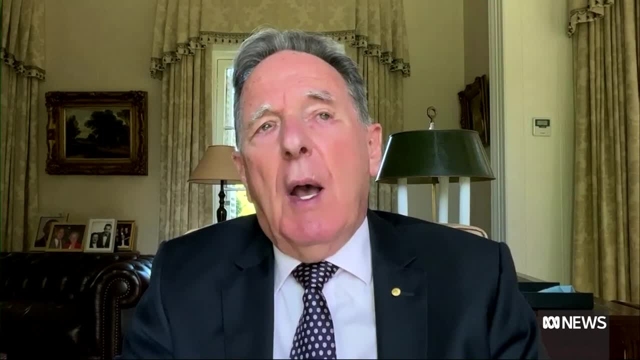 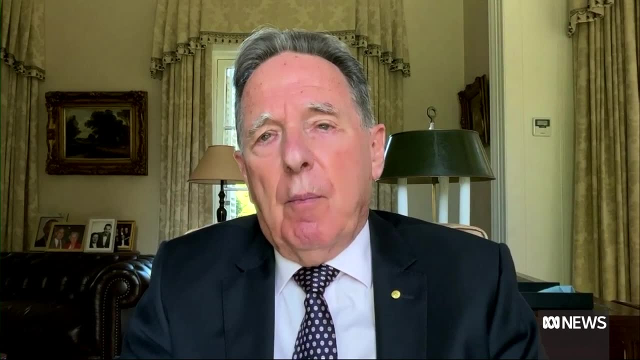 oversight by the Environment Protection Agency and, as well, will be subject to the disciplines that are imposed by national environmental standards. Graeme Samuel, we really appreciate you taking the time to speak to us. Thank you, Thank you.